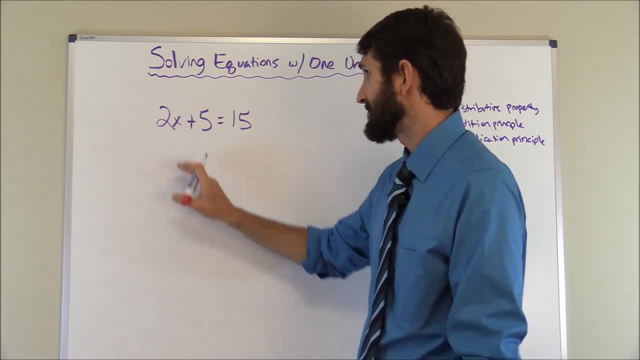 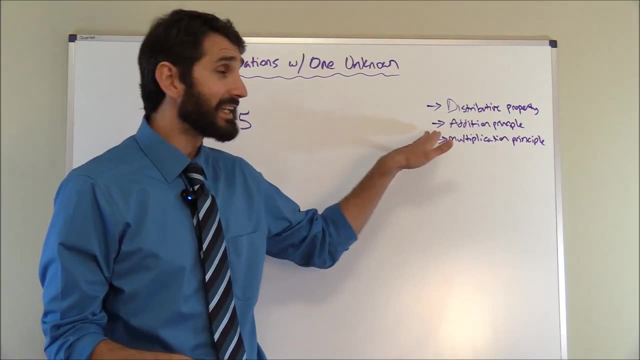 side. So, in order to do this, the first thing that I see here is that it's a plus 5.. Now, anytime you have just a number like plus 5 or minus 5 or something like that, you can use a rule called the addition principle. What is the addition principle? Well, basically the addition principle. 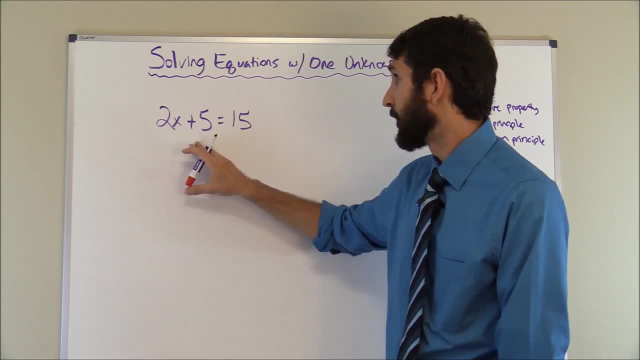 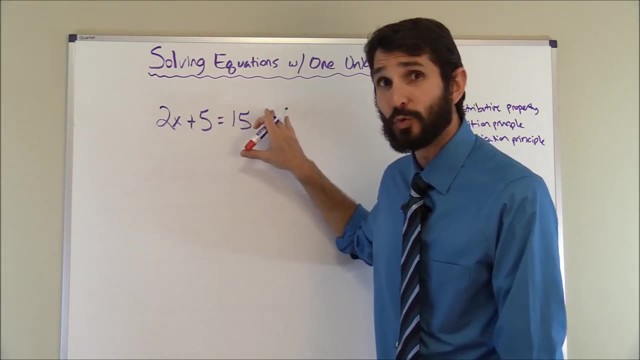 just states that whenever you have a plus number or minus number, you can do the opposite on this side of the equation to cancel it out. but whatever you do to this side of the equation, you also have to do to the other side of the equation. So basically, you're manipulating the number plus. 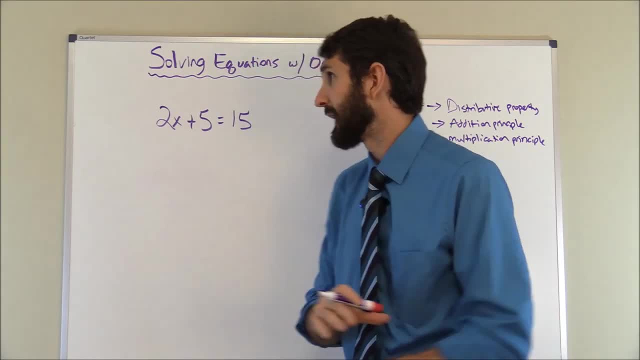 the equation around. It's going to remain the same. You're just manipulating it to find out so you can solve for x. So in this case we have 2x plus 5.. What we're going to do is we're going. 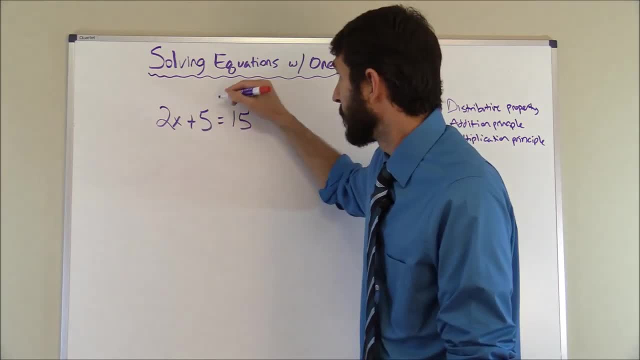 to apply the addition principle to say, since that's a plus 5, we're going to say minus 5 because we want to cancel that out. So we have a plus 5.. We're going to take 5 away, We'll have. 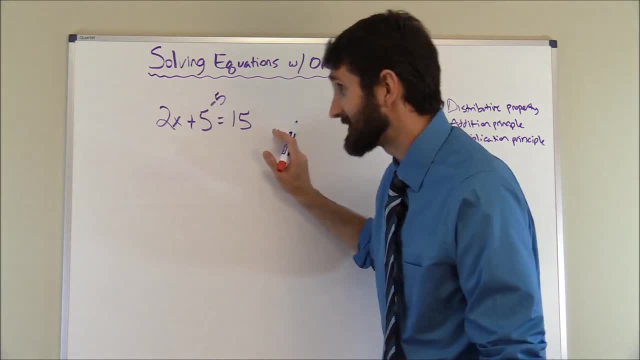 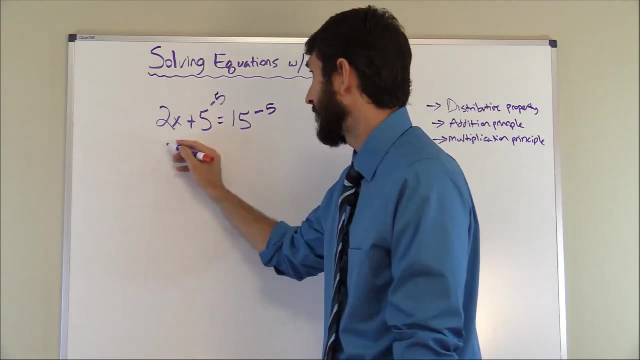 nothing on this side, But what we do to this side, we got to do to this side. So since we said minus 5 here, we've got a minus 5 here, Okay, so let's carry our problem down. Now we're going to. 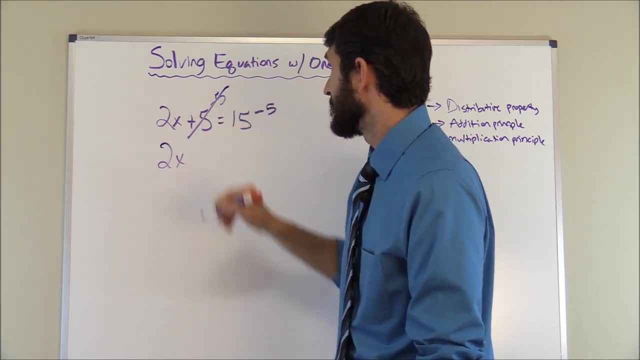 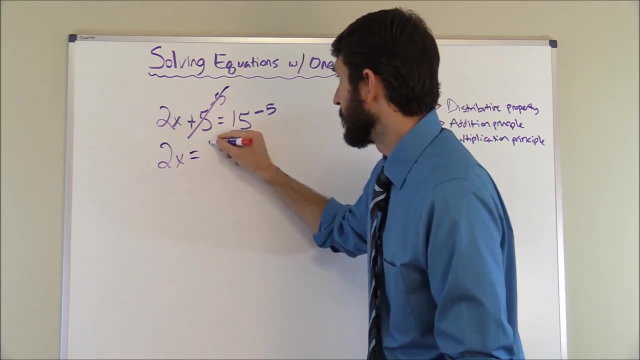 have 2x This canceled out, so we have nothing left there to carry down. equals 15 minus 5 is what It's 10.. So 2x equals 10.. Okay, we're getting close. now We almost have our variable. 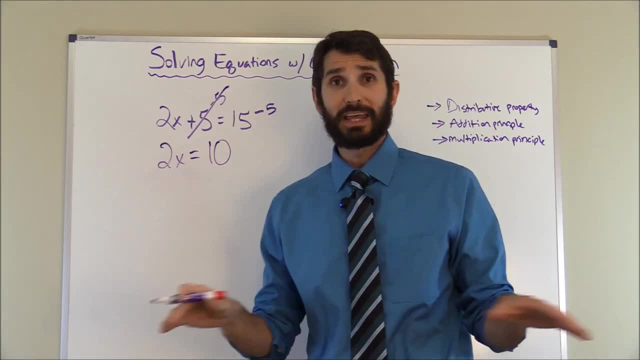 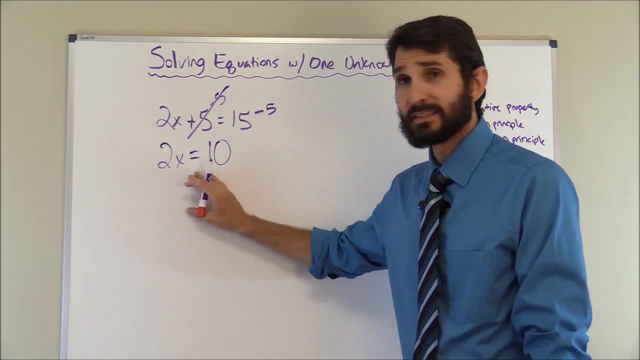 and our number, but we have a 2 in front of it and we got to get rid of that 2 because we want to end with just what x by itself stands for. So, in order to simplify this and solve this down even further, what we can do is we can use another. 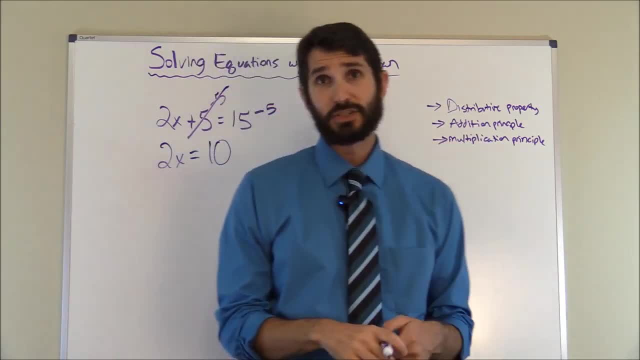 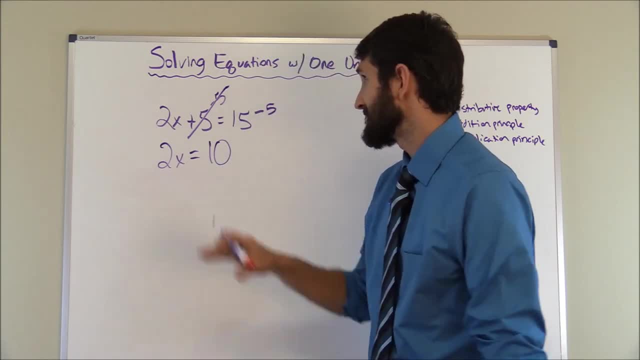 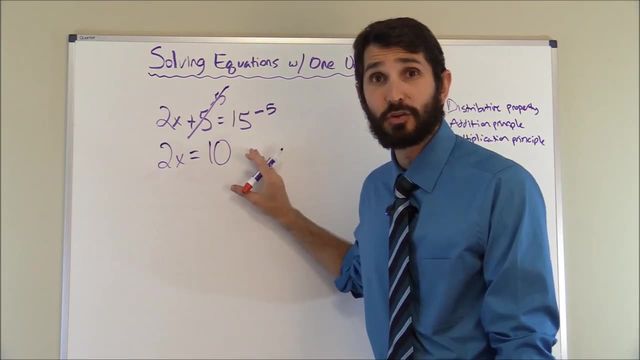 principle And the multiplication principle basically states the same thing: You can multiply or divide on one side of the equation, but what you do to one side, you have to do to the other side to keep the equation balanced. So what we're going to do here? we want to get rid. 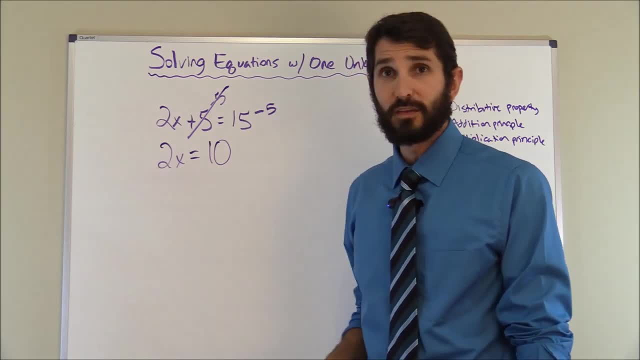 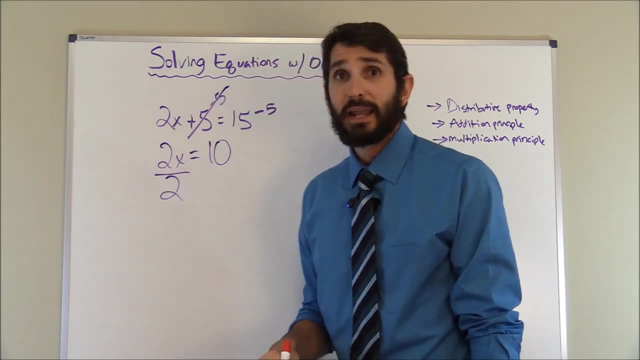 of this 2, and it's 2 times a number. In order to get rid of the 2, we're going to divide it by 2.. So that's how we're going to get rid of it. We're going to just put that over 2.. Now what we? 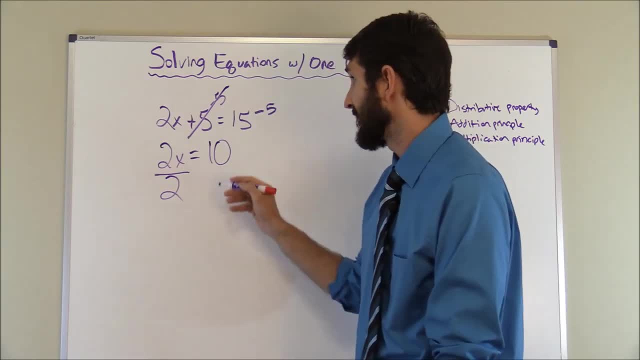 do to one side of the equation, we got to do to the other side. That's what the rule states, So it's going to be equals 10 over 2.. Now we can go ahead and simplify this a little bit, because 2. 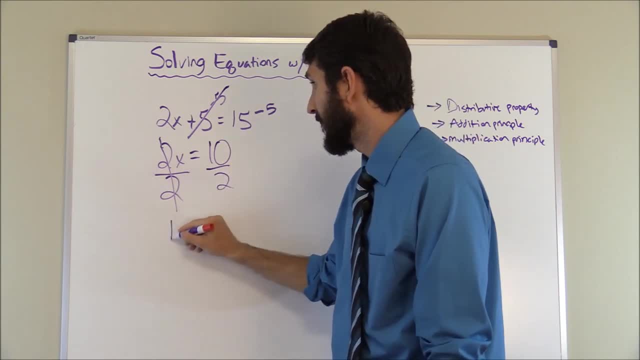 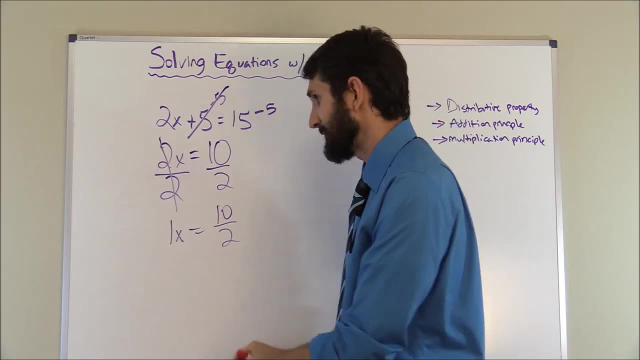 divided by 2 is going to cancel out and that's going to give us a 1x equals 10 over 2.. Now, whenever you have a 1x, that's the same thing as saying just x by itself, So it's usually helpful. 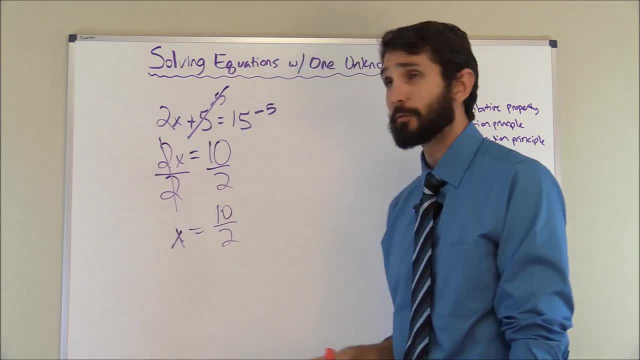 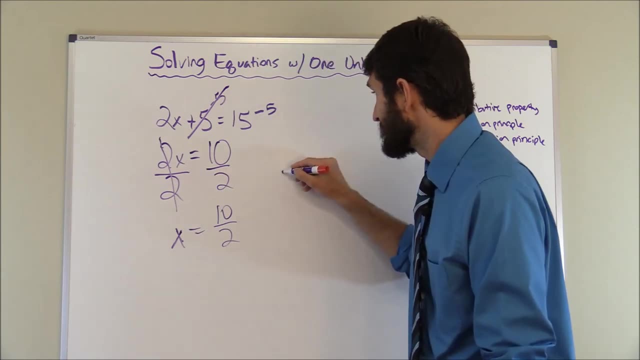 just to get rid of that, so you don't get confused. So it's just going to be: x equals 10 over 2. And that's basically our answer. but because this is an improper fraction, we could go ahead and simplify that even more, because 10 divided by 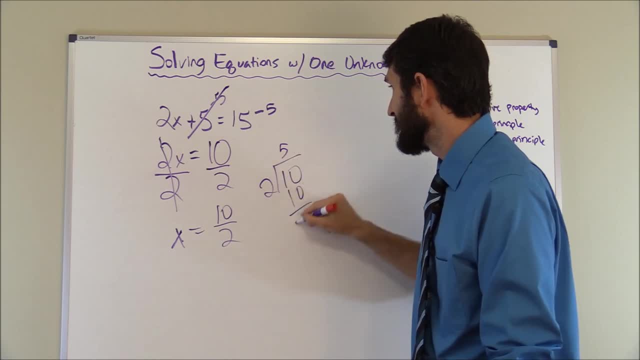 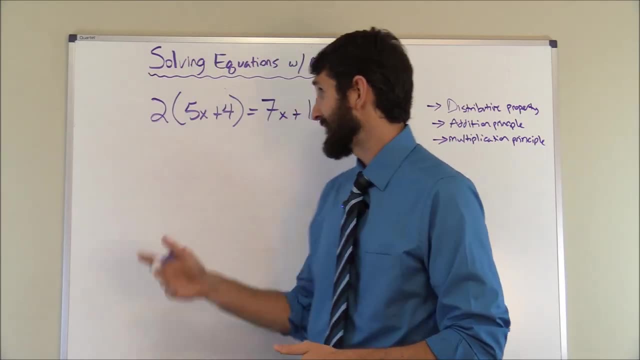 2 is going to be what? 5.. 2 times 5 is 10.. So, basically, x equals 5 is another way to simplify. Okay, now let's work another one of these equations And, as you will see, this one looks. 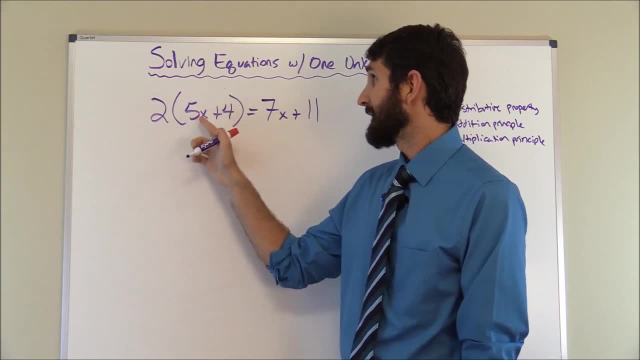 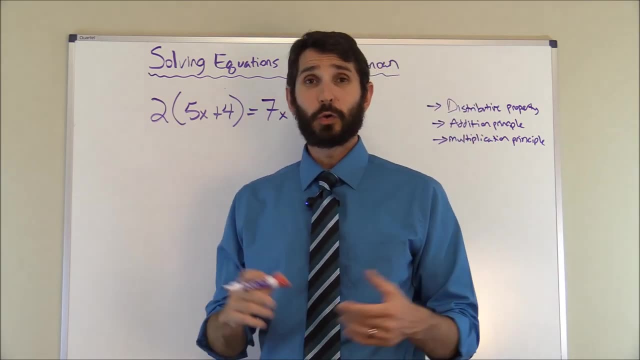 a little more complicated. It's 2 times 5x plus 4. in parentheses equals 7x plus 11.. And again, it looks complicated, but it's not going to be that bad. We're going to get through this by using a few simple rules here, And the first thing we're going to want to do is get rid. 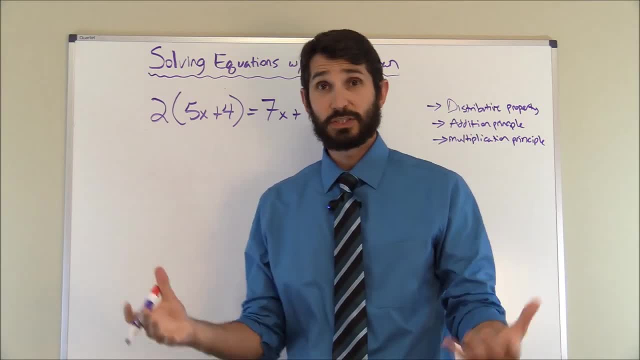 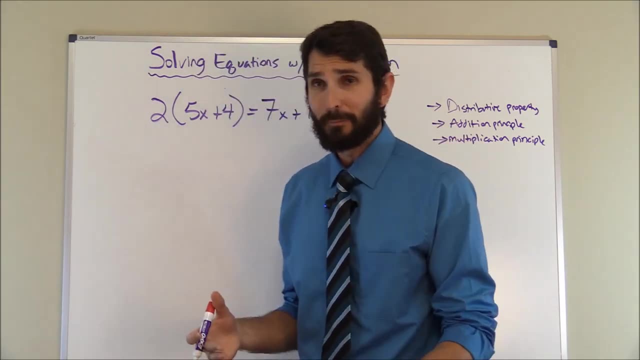 of this parentheses, because that makes it look complicated, And so let's just go ahead and solve that first, because that's what we need to get rid of, And to do that we use something called distributive property, And all that means is basically, you multiply this number here times. 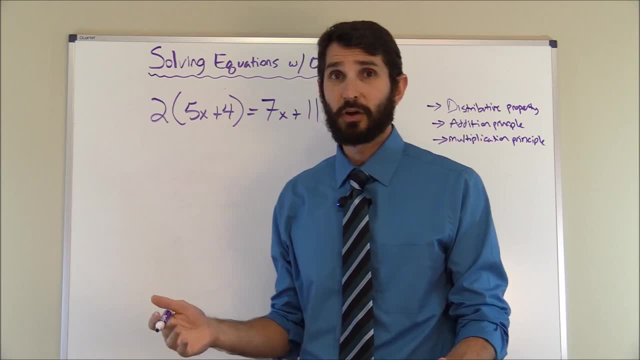 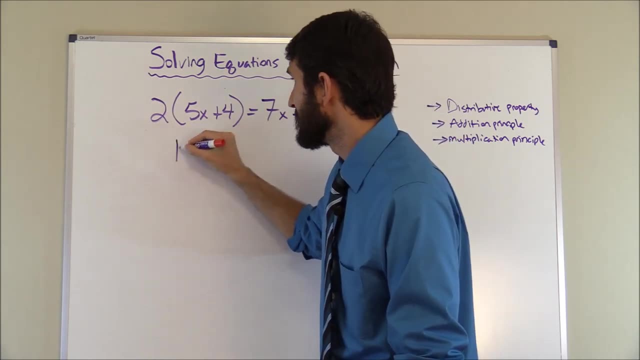 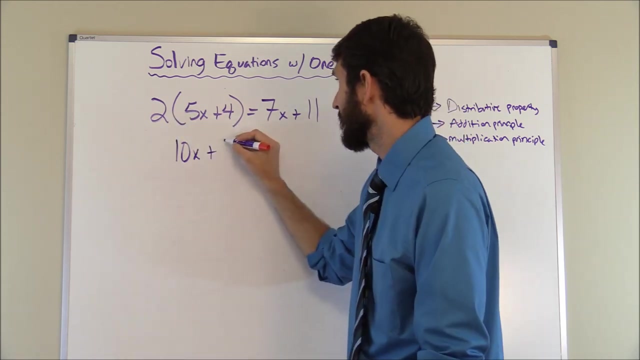 this and then multiply that number, times that and carry it down and you'll have your answer. that will get rid of the parentheses. So what we do is we say 2 times 5x, that's going to give us 7x, plus 2 times 4 is going to give us 8.. So we just carry that down, So it's going to turn into: 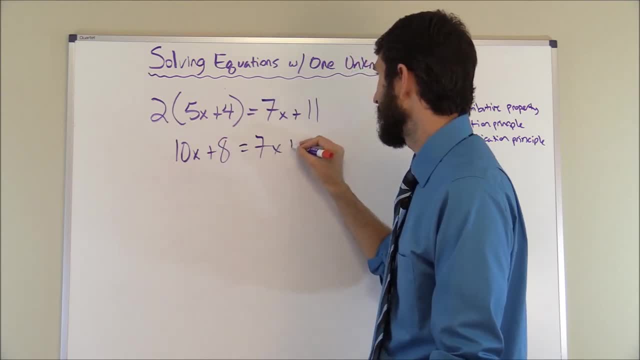 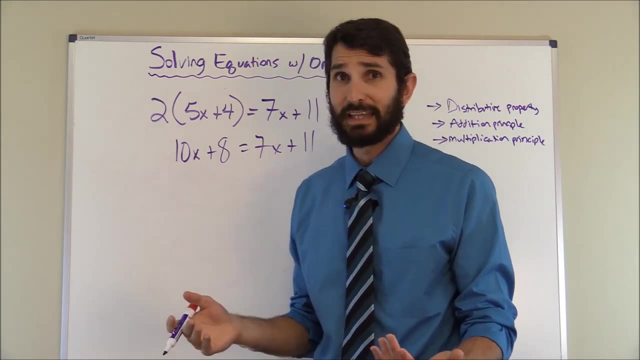 10x plus 8 equals- and we'll go ahead and carry this down- 7x plus 11.. Okay, now we're going to go ahead and attack these numbers here, because again, those are the ones I like to get rid of. 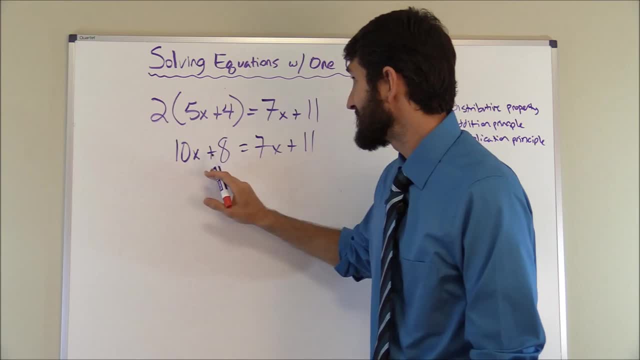 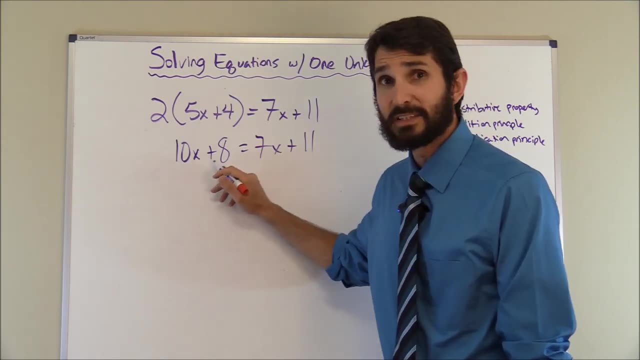 first, And we do that using the addition principle, which states that we can do the opposite of the number here to get rid of it on this side of the equation. but we got to do the same here, So it's 8.. So how do we get rid of a plus 8? We subtract 8.. So we're going to subtract 8 from this side. 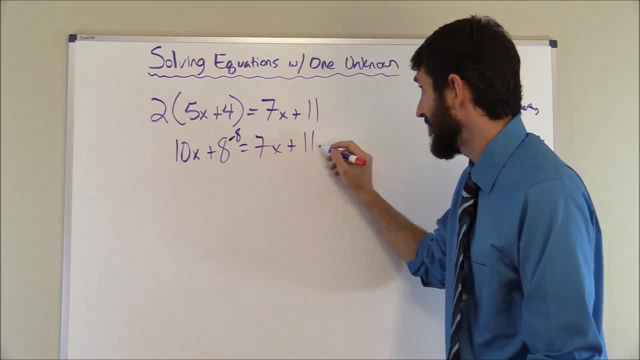 What we do here, we got to do here. So we come over here to the number on this side, and it's plus 11.. So we're going to say 11 minus 8.. Okay, now let's go ahead and carry this down, So we're. 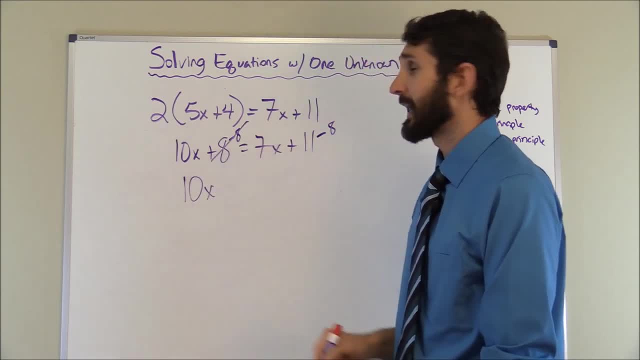 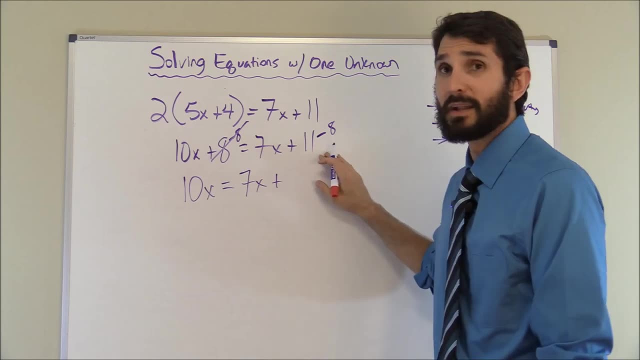 going to have 10x plus 8 minus 8.. Those cancel out. We're going to have nothing to carry down there. We just put our equal sign and it's going to be 7x plus what's 11 minus 8? That's going to. 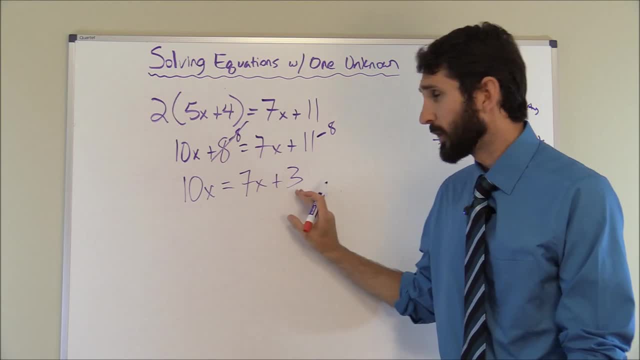 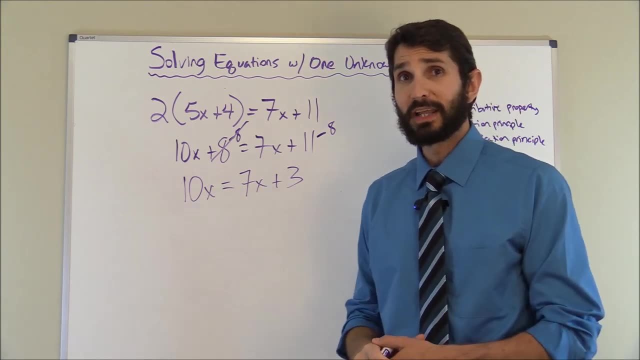 give us 3.. Okay, so we just carry that down. So we're going to carry that down, So we're going to just have one number left. but we have two of these coefficients here, with a coefficient and a variable. Now, how are we going to get rid of this? Well, in order to get rid of this, we're 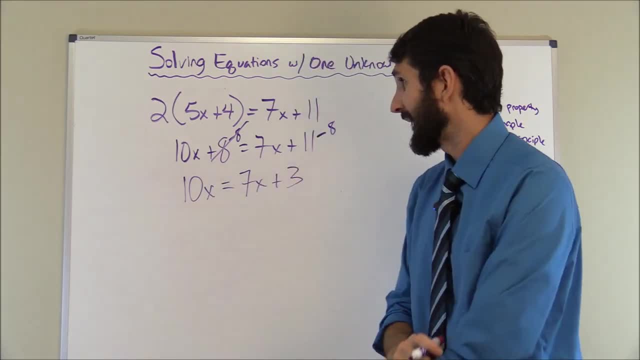 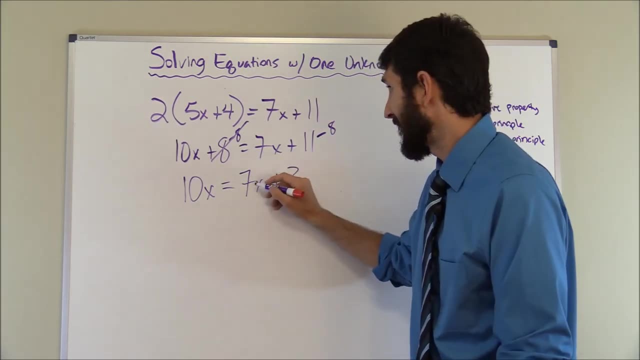 going to use again the addition property. We're going to take 7x and try to move that to the left side because we want the variables and then the numbers. So in order to do that- again the addition principle- we have a positive 7x. So we're going to subtract 7x. But what we do here, 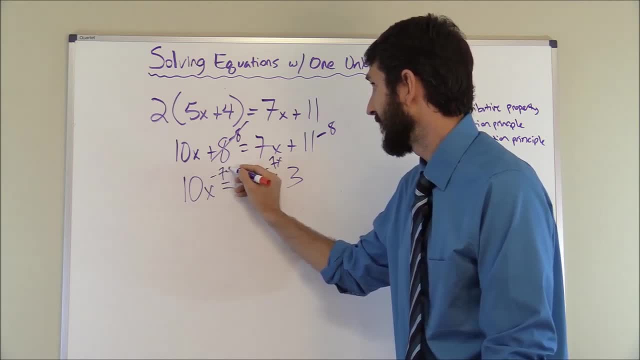 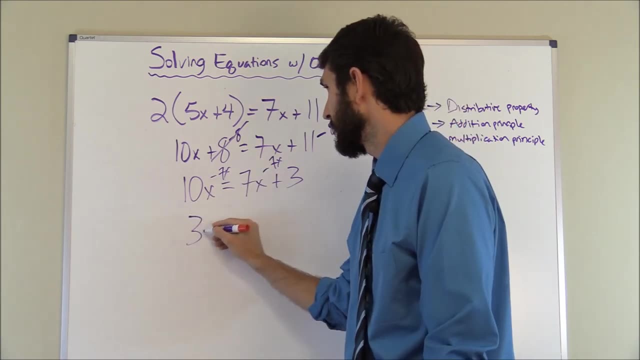 we got to do here, So it's going to be 10x minus 7x. Okay, so we'll go ahead and carry that down. 10x minus 7x is going to give us what? 3x, So 3x. 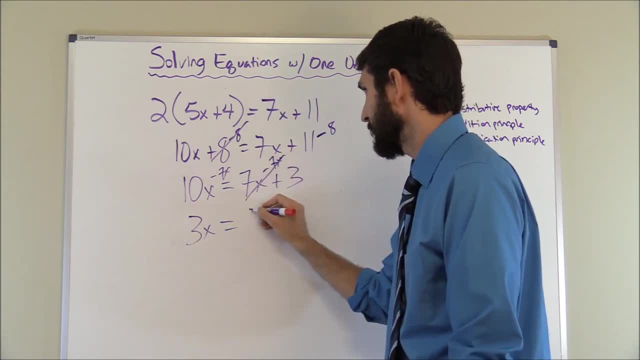 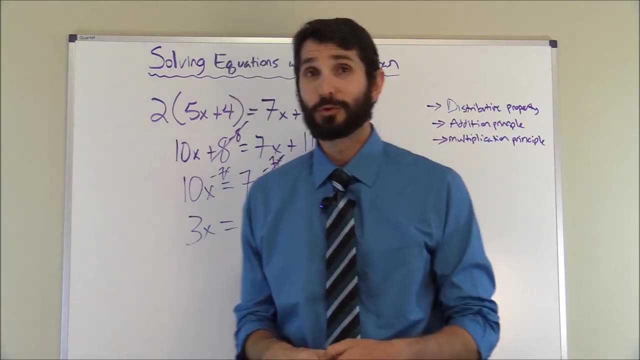 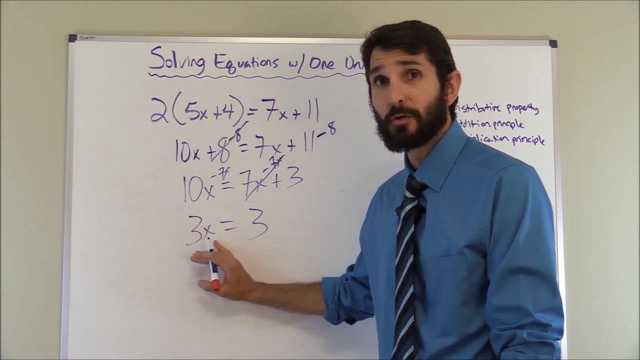 equals. that's canceled out now and we have just a positive 3 left over. So we're going to have 3x equals 3.. And now we can use the multiplication principle to go ahead and finish this so that we just have an x left And what we do, it's 3 times a number. So in order to get rid of it, we're 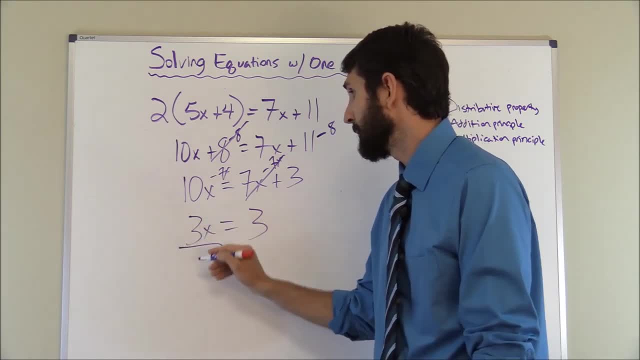 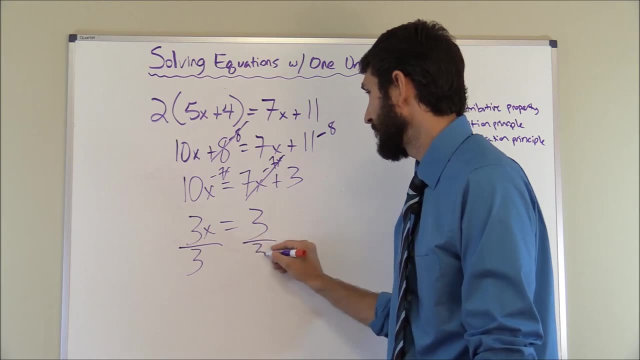 going to do the opposite, which is divide. So we're going to divide that by the number here, and we got to do it to the other side, because what we do to one side we got to do to the other side. So it's going to be 3 divided by 3.. So those 3s will just basically cancel out. We'll have an x. 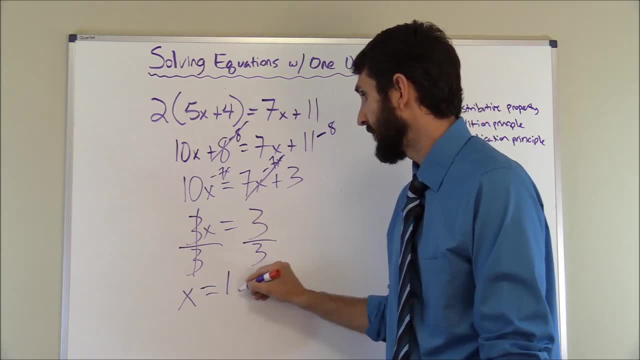 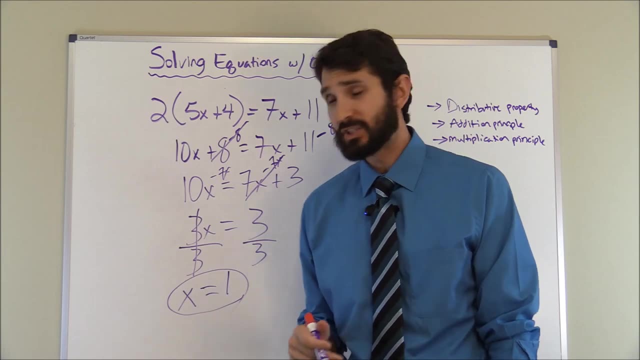 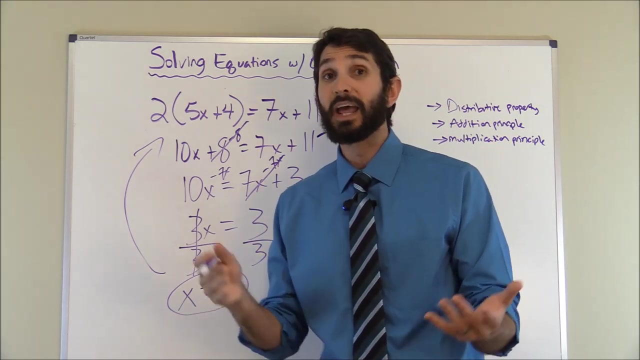 equals 3, divided by 3 equals 1.. So our answer is x equals 1.. Now I should go ahead and stop right here and tell you that the cool part about these types of equations is that you can take the final answer and go back and substitute it in the original equation to see if it works out right. 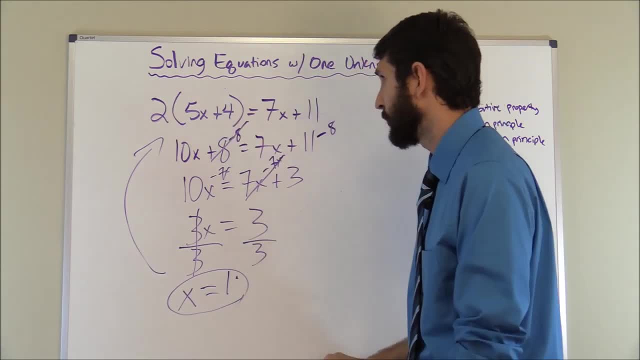 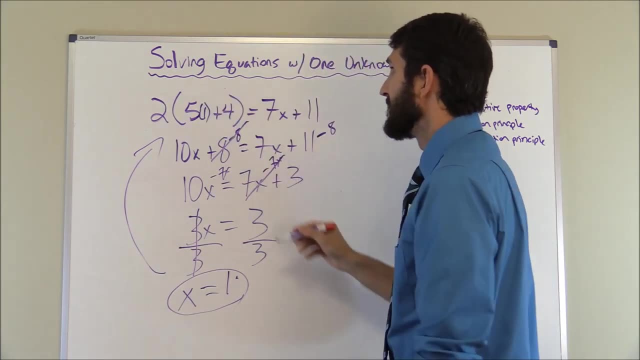 This is a way you can check yourself. So let's substitute 1 where the x is here, which would be 5 times 1.. And let's see if this works out. So we start with the parentheses. 5 times 1 is 5 plus 4. 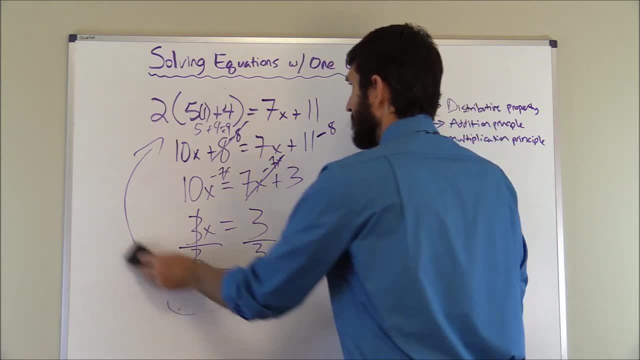 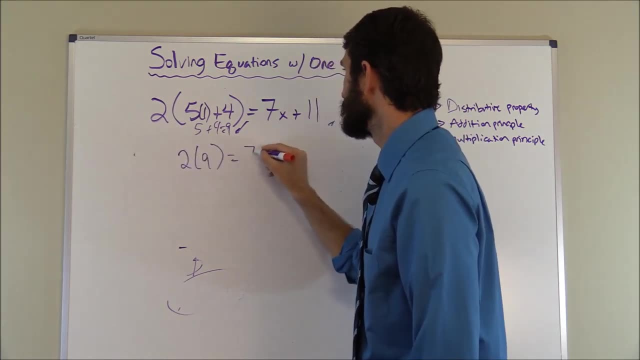 equals 9.. I'll erase this here, And so what we're going to have is 2 times 9 equals 7 times 1 plus 11.. Okay, 2 times 9 is going to get us 7 times 1 plus 11.. So we're going to have 2 times 9 equals 7 times 1 plus 11.. 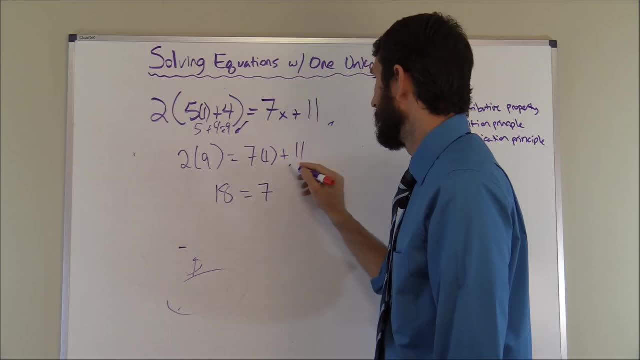 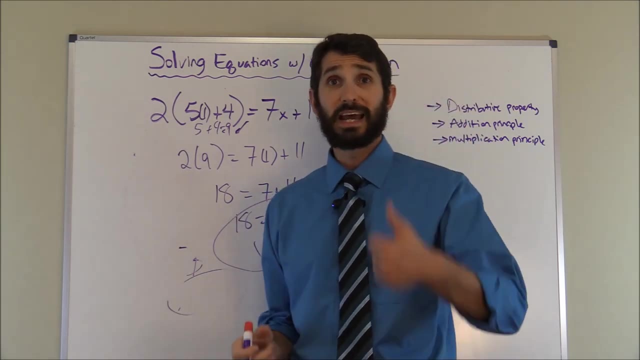 Give us: 18 equals 7 times 1 is 7 plus 11.. So 18 is going to equal 18.. Does that sound right? Absolutely, We are done. It checks out. So we are good to go. Okay, now let me show you one of these. 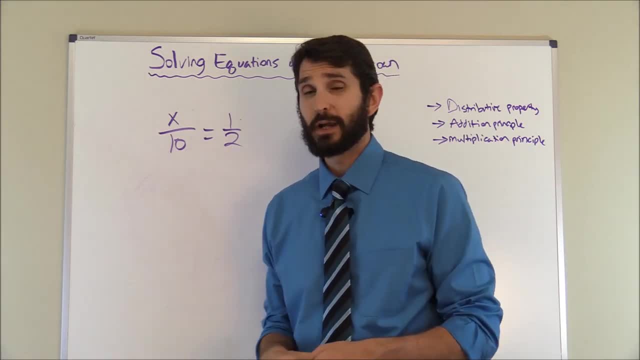 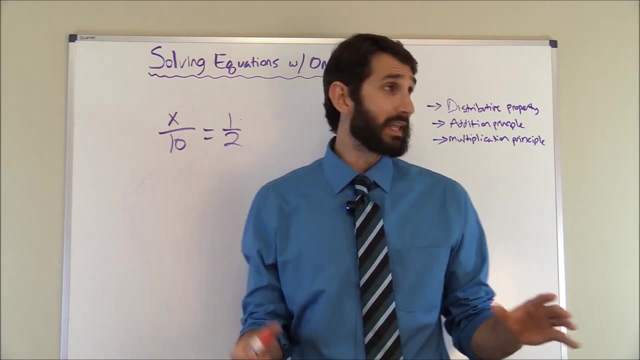 in fraction format, so you can get a hang of that, because they will have these in fraction format sometimes. So here I have: x over 10 equals 1 half, And this looks a little bit complicated, But again, if we just follow these simple rules, you'll find out that it's actually quite easy. So if you'll remember, in the last video we said that we were going to have x over 10 equals 1 half. So we're going to have: x over 10 equals 1 half. So here I have: x over 10 equals 1 half. So we're going to have. 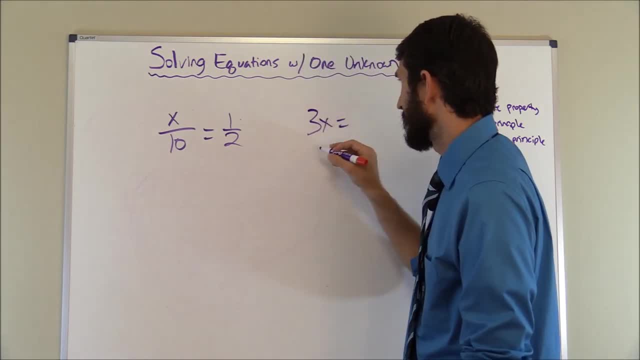 x over 10 equals 1 half. So we're going to have x over 10 equals 1 half. So we're going to have something like this. There was like a 3x equals whatever the number was, And I told you that to. 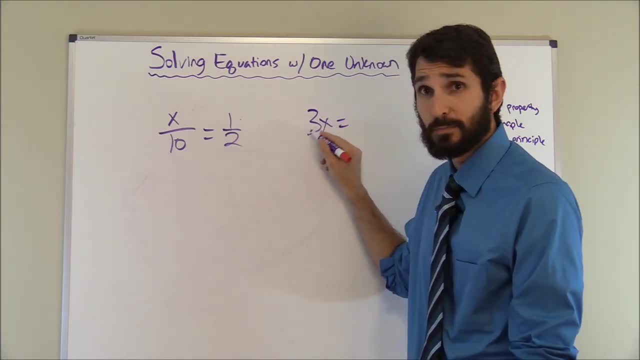 get rid of this 3 so that you just have an x. what you need to do is, since it's multiplication right here, 3 times x, you just simply divide by 3. And that's going to cancel out the 3 and just leave. 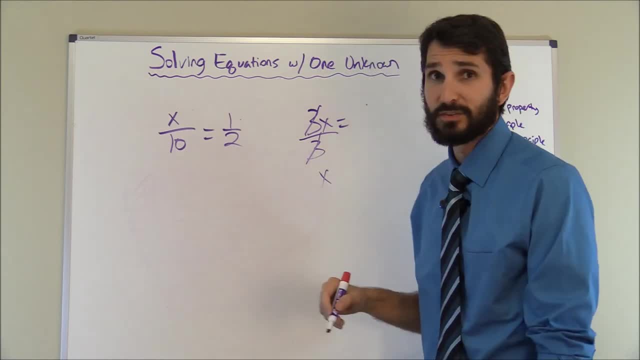 you with an x equals, But you had to also do it to this side as well. You had to divide whatever number was here. If it was a 3, you had to divide that by 3 as well. Well, it's the same principle. 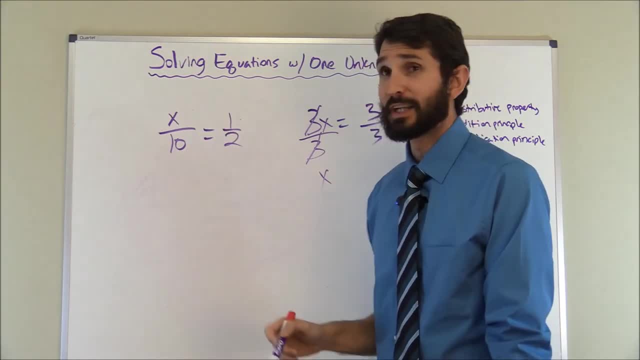 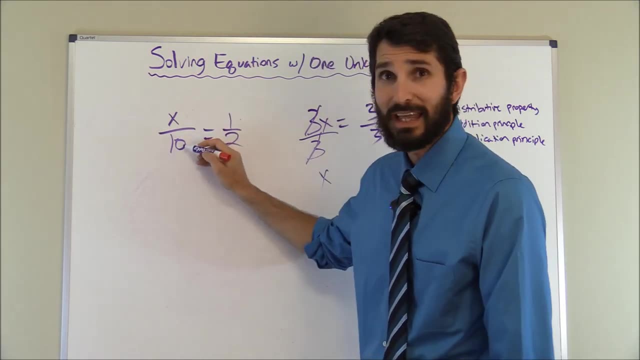 here We're going to apply the multiplication principle, But since it's division, what we're going to do is we're going to do the opposite, which is multiplication. So in order to get x isolated here, we're going to need to cancel this out. So all we do is we multiply the top by. 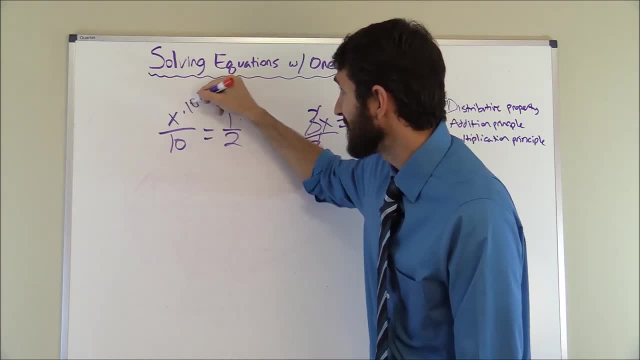 whatever's on the bottom. So it's an x. We're going to multiply that by 10, because now you'll see we have a 10 here and a 10 here, And 10 divided by 10 is going to give you 1. It's going to cancel. 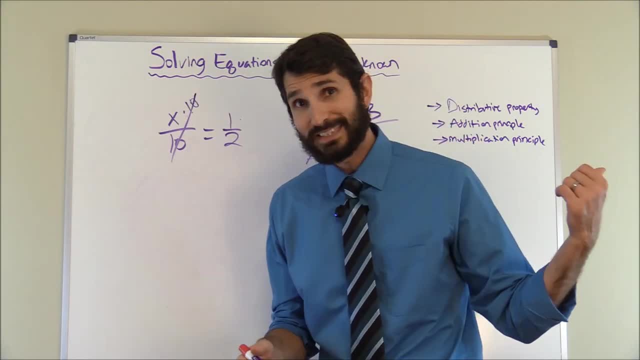 it out and we'll just have that x left. But again, what you do to one side you got to do to the other. So we have 1 here. We're going to have to multiply that by 10 on this side, So we'll go. 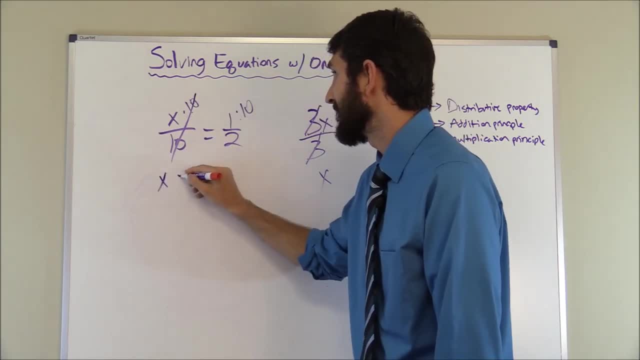 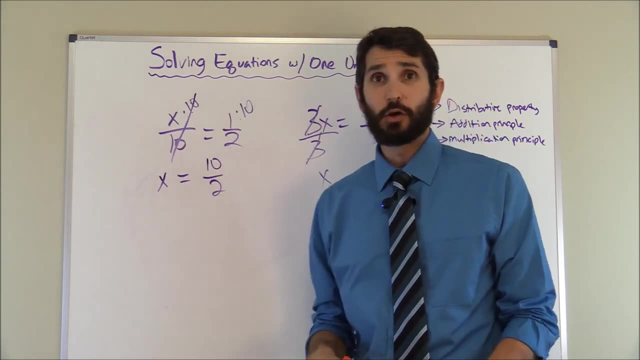 ahead and carry this down Again. the 10s cross out. We have an: x equals 1 times 10 is 10 over 2.. Now our answer is x equals 10 over 2.. But we could simplify this even further, because 10 can be divided by 2. 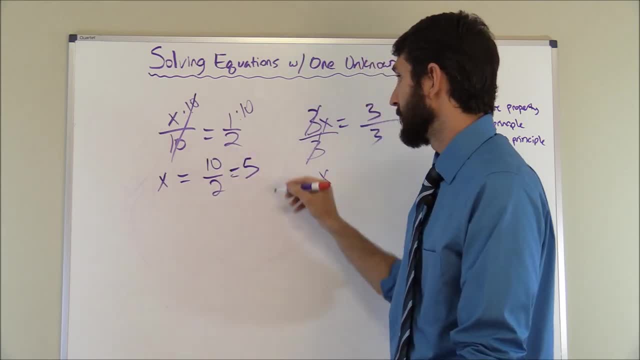 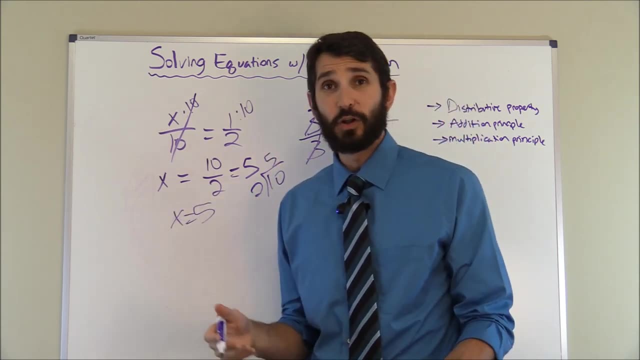 equally, which will give you 5,, a whole number. So because 10 divided by 2,, 2 will go into 10 five times, So our answer is: x equals 5.. Now again, you can always double check your answer. 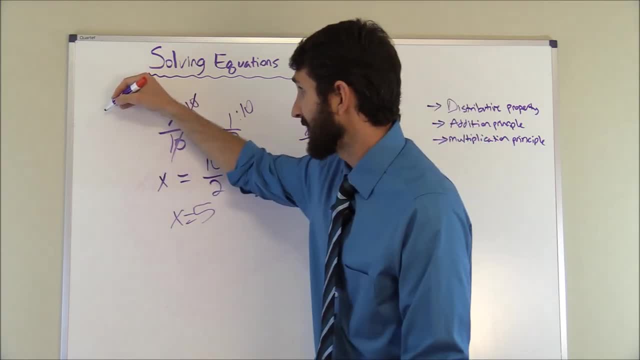 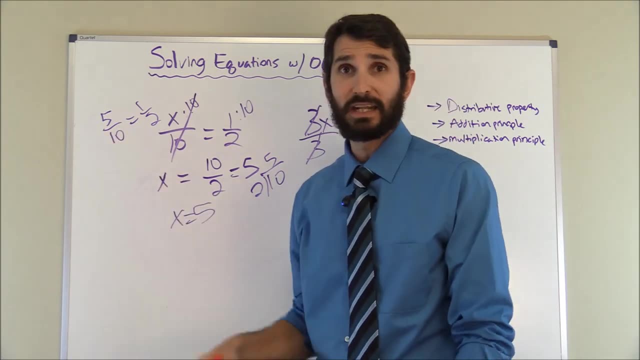 by putting that in here to make sure it works out. So x over 10 will put the 5 where the x was 5 over 10, does that equal 1 half? Yes, because 5 over 10 can actually be reduced to 1 half if you simplify that. So 1 half equals 1 half. 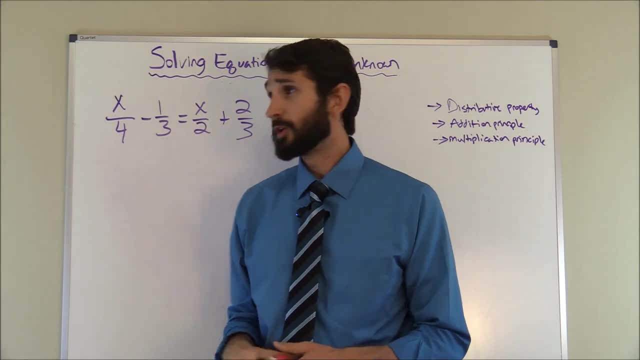 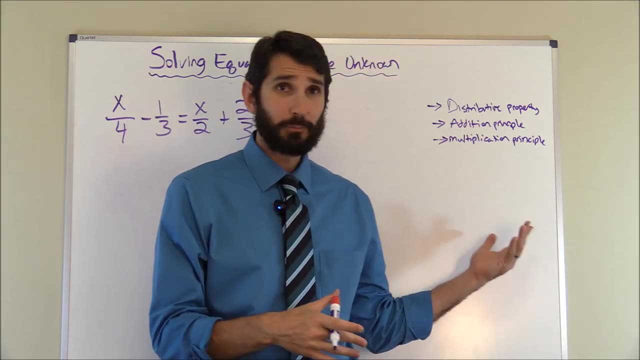 Our equation checks out. That's how we solve that. Okay, now I'm going to do a slightly more complicated fraction type equation to show you how this works. And again you use the exact same principles. We don't have any parentheses, so we don't have to worry about doing that distributive. 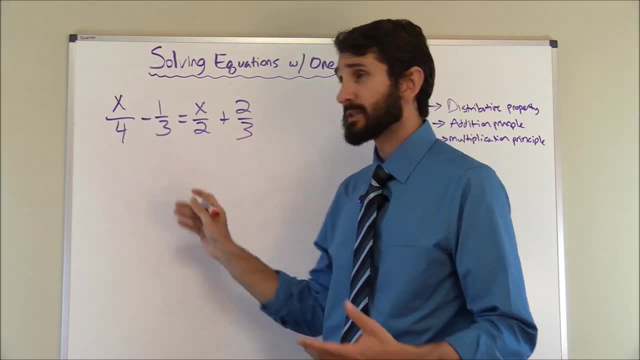 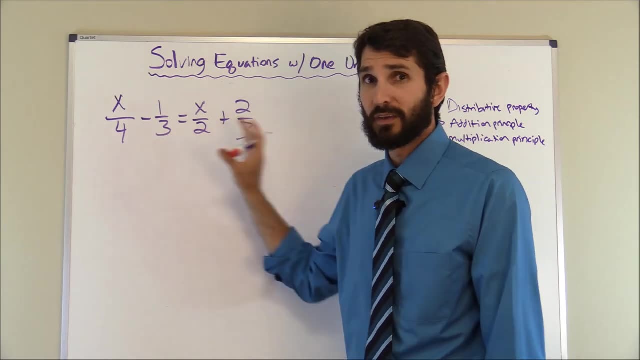 property thing. But we do have the variables and the numbers and we're going to get the variables on one side and the numbers on the other side. So I always like to start with the number part, because that's just a little bit easier. Let's begin to work the numbers to the right and the variables to the left. 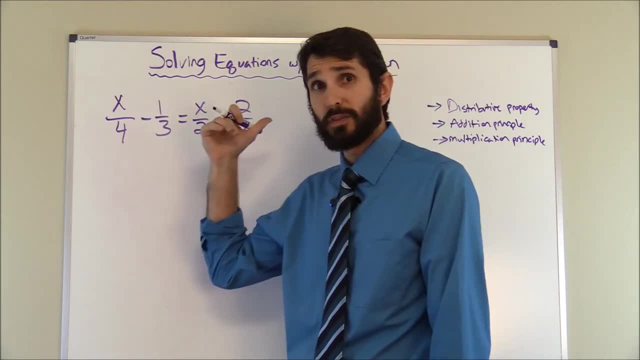 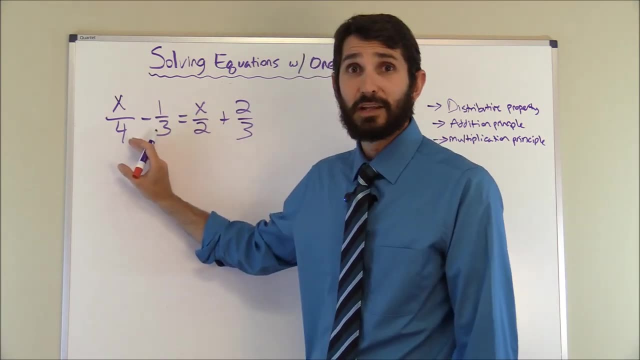 So we have x over 4 minus 1 third. We want to get the 1 third to the other side of the equation. How do we do that? The addition principle, which states that we do the opposite to one side to get rid of the number. But whatever we do here, we got to do here. So this is x over 4 minus 1 third. 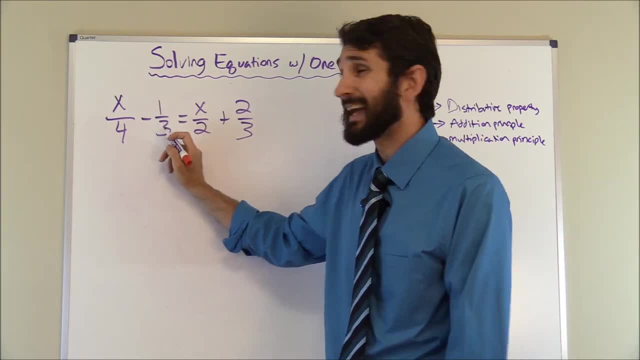 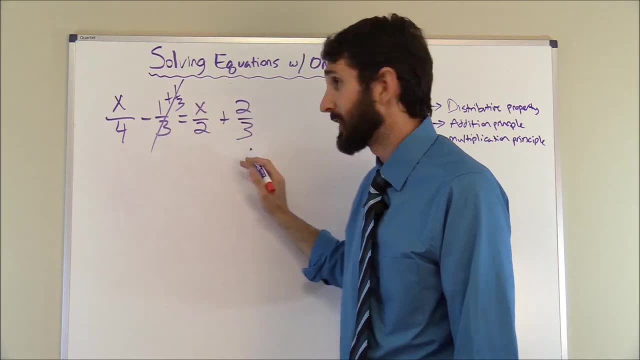 What's the opposite of minus 1? Positive 1 third. That's how we're going to get rid of it here. So we add 1 third so that we can cancel that out. But what we do to one side we got to do to the other. We can't be greedy, So we're going to 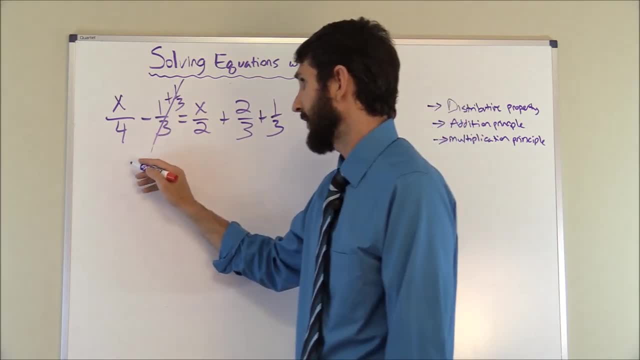 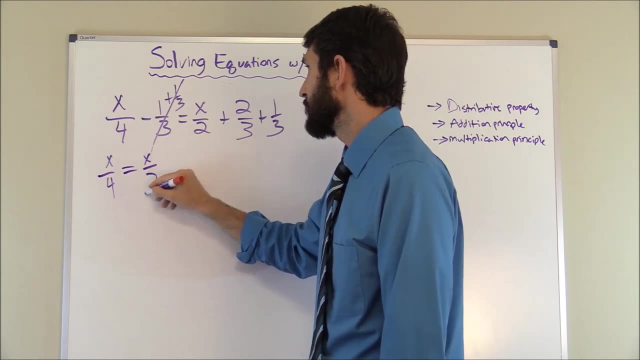 add 1 over 30 here. Now we'll go ahead and carry this down. It's going to be x over 4.. We eliminated that, so we don't worry about that. Equals x over 2, plus now we have 2 thirds and 1 third Now I. 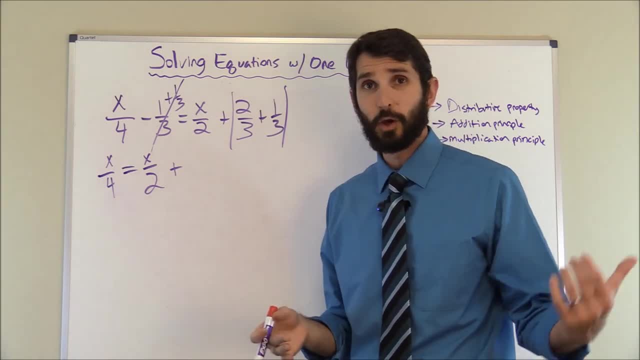 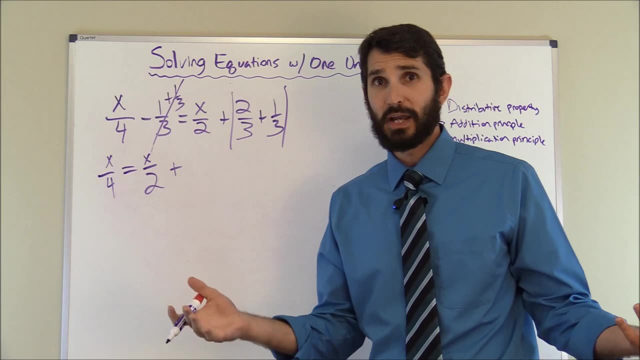 did a video on adding and subtracting fractions so if you're a little fuzzy on that you can go back and check that video out. But whenever you add and subtract fractions you always want to make sure the denominator is the same. You can't just add and subtract fractions as they have different. 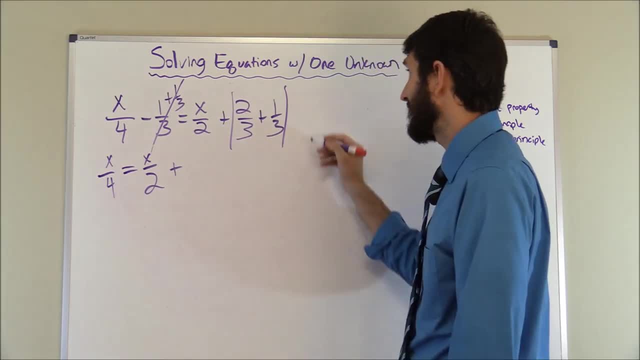 denominators. In this case they are the same, so we can just go ahead and add that. And how you do that? you just carry the denominator over, which in that case is the 3, and then you add the numerator. So 2 plus 1 equals 3.. So it's 3 over 3, or another way to say that is just simply 1,. 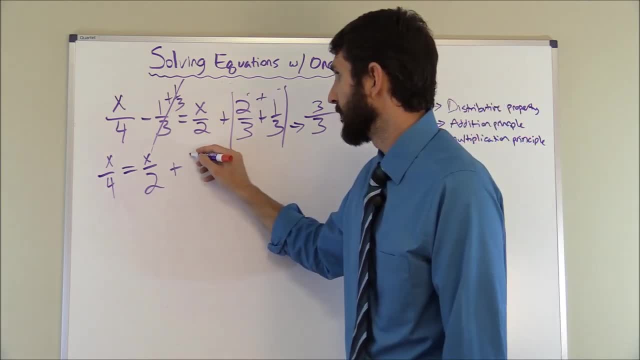 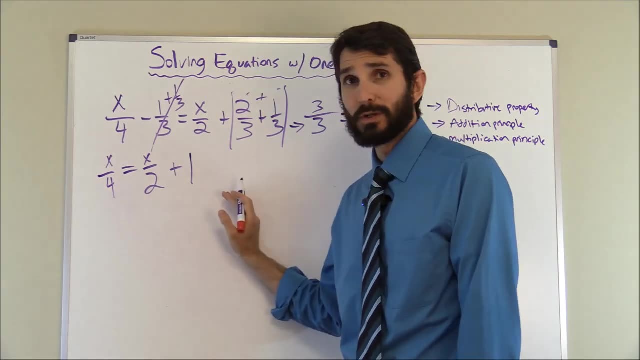 because 3 divided by 3 is 1.. So it's x over 2 plus 1.. Okay, Now we're going to try to get this x over 2 to the left side, so we have number on one side and all our variables on the other side. How do we do that? again, The addition principle, because it's 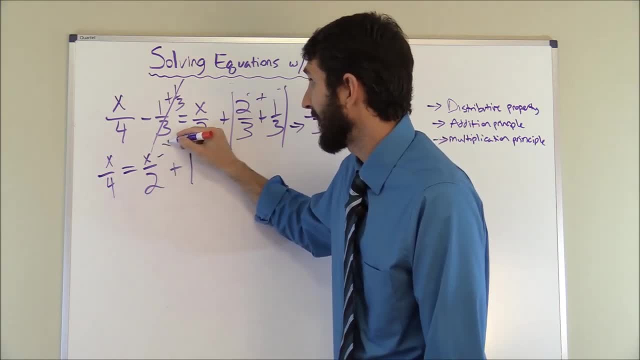 a positive x over 2.. So what we're going to do is we're going to subtract x over 2.. That's going to help us get rid of that. But what we do to one side we got to do to the other, So that's going. 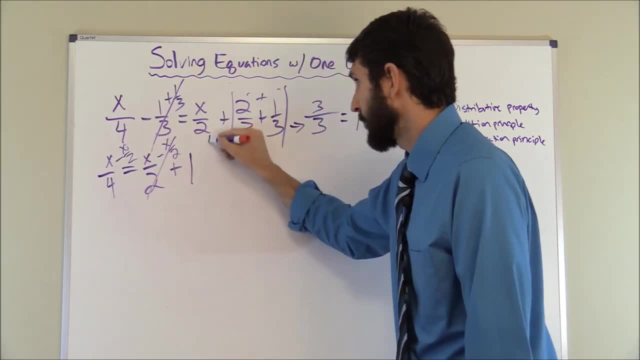 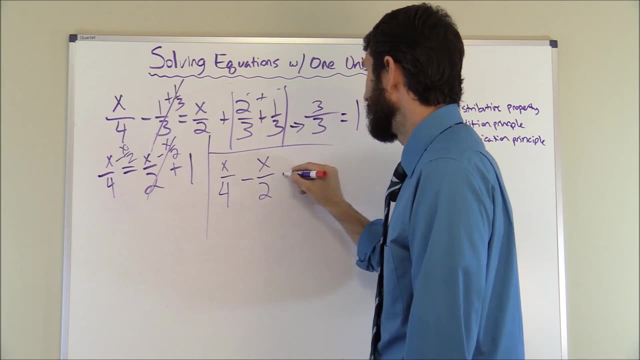 to be minus x over 2 on this side as well. So we'll just go ahead and rewrite that here. That's going to be x over 4 minus x over 2.. So that's going to be minus x over 4 minus x over 2 equals 1.. Now, we can't subtract these fractions. 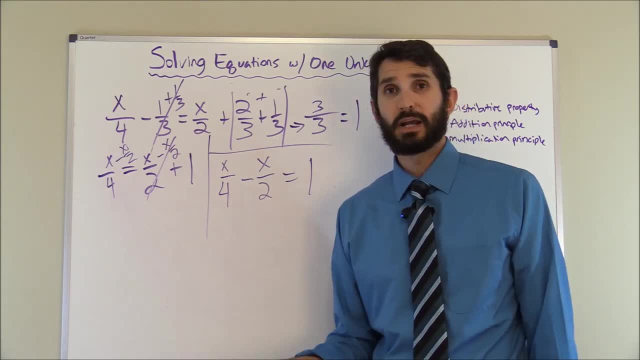 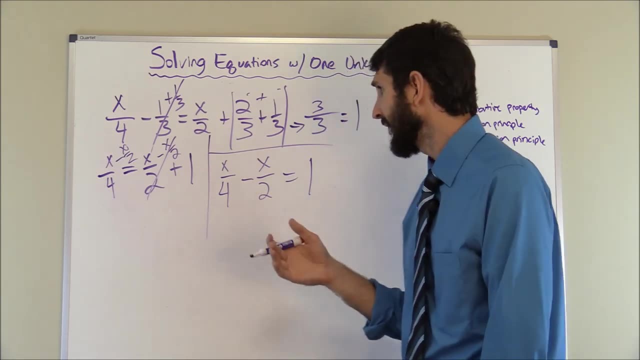 because they have different denominators And, like I just said, we can't just add and subtract fractions if they have different denominators. So in order to proceed with this problem, we have to find the least common denominator here And whenever you find the least common denominator, 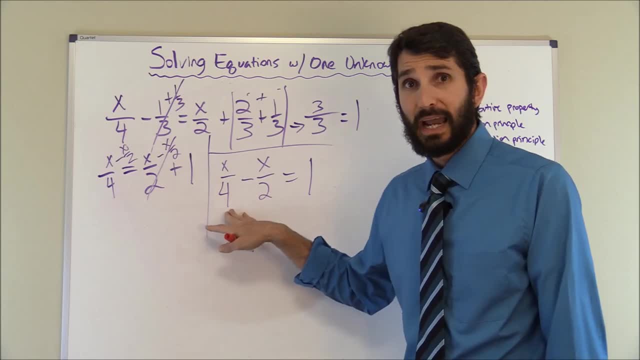 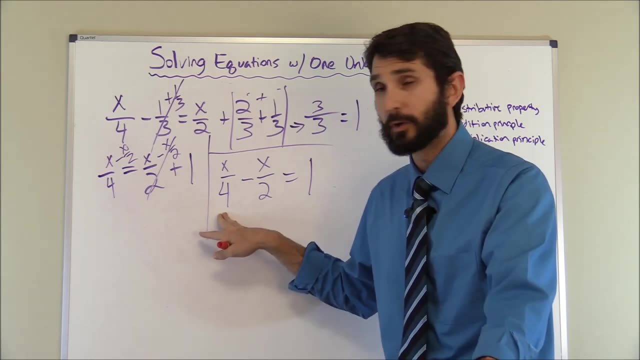 the easiest way for me is I look at the bigger of the two and I just first ask the question: will the smaller denominator actually multiply into that larger denominator evenly and produce a whole number? And if so, then that's your least common denominator, And if not, you begin to multiply this larger. 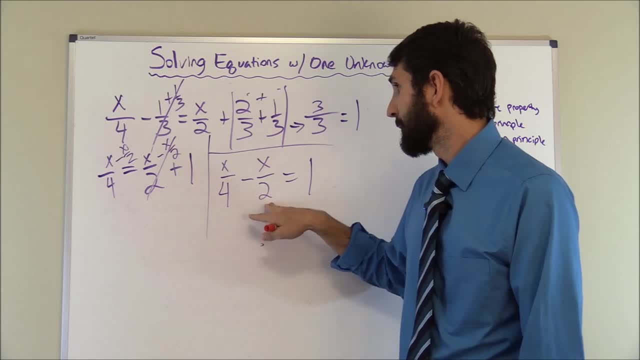 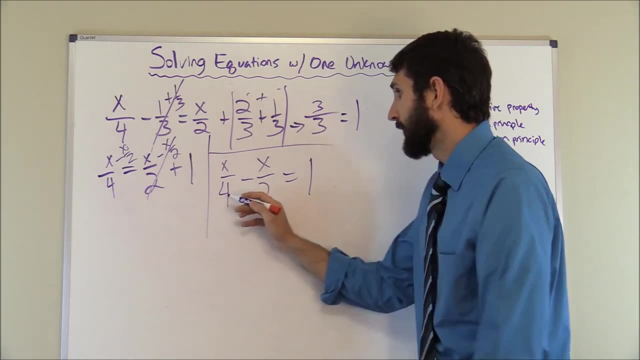 number by 2, by 3,, by 4,, until you'll find a number that both this will multiply into and that will multiply into. In this case we're lucky because 4, will 2 go into 4 evenly. Yes, So our least common. 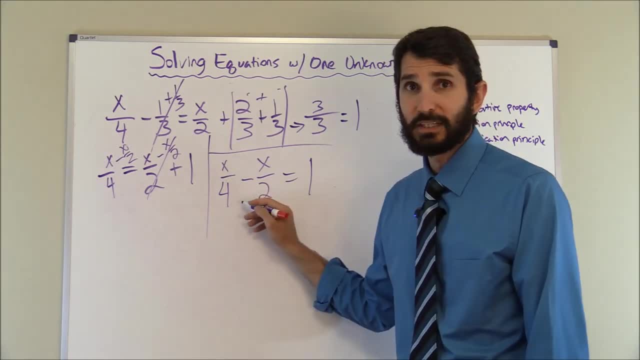 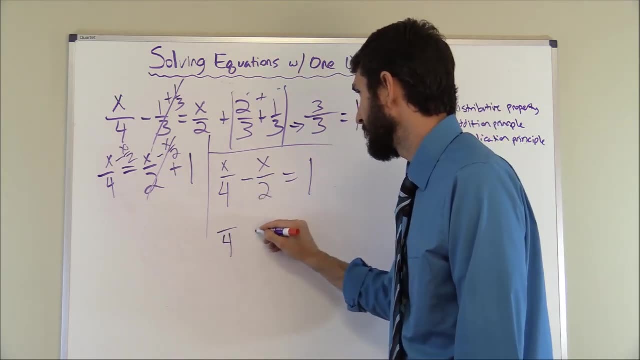 denominator is actually going to be 4.. So let's go ahead and convert these fractions out and get the common denominators here. So what we're going to do, the new denominator is going to be 4 for both of those fractions, because that's the least common denominator, And then we're going to 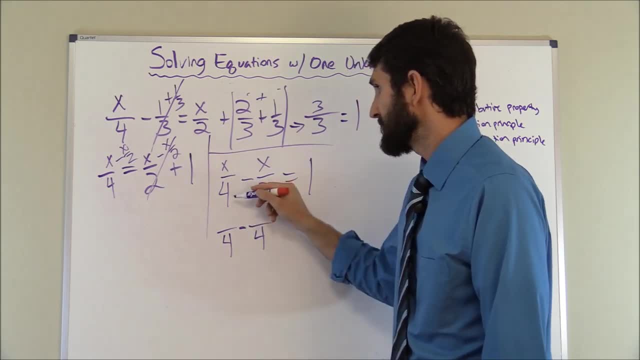 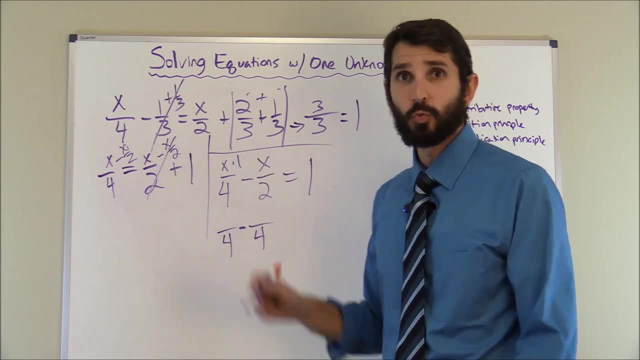 separate that that's the least common denominator And it's going to be a minus sign. So what we'll say is: 4 will go into 4, how many times 1.. You multiply 1 by the numerator X times 1 is going to be 1x, or. 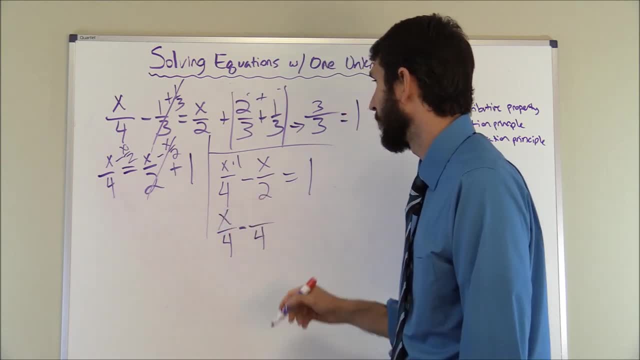 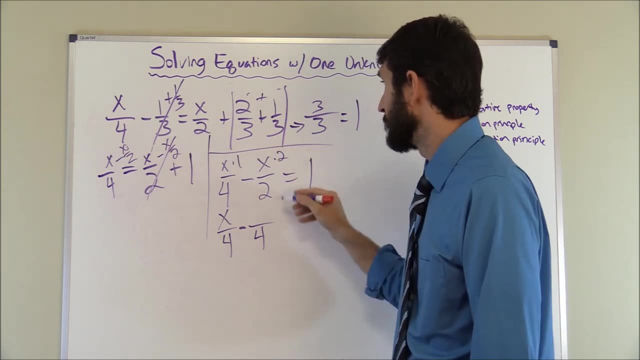 another way of saying that is just simply x, So it's going to be x over 4.. 2 will go into 4 times. or 2 will go into 4, how many times 2.. So we multiply X times 2.. 2 times X is what It's: 2x. So it's going to be 2x. there equals 1.. 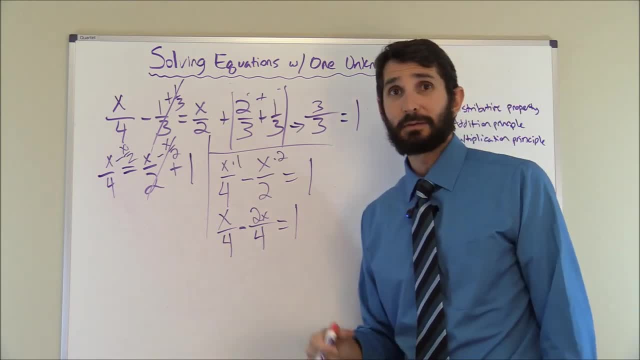 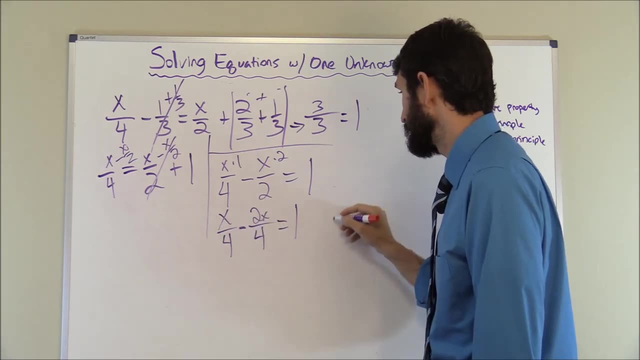 We carry that 1 down. Okay, now the denominators are the same and we can go ahead and subtract this out. So 1x minus 2x is going to give us negative 1x. So it's going to be negative x or 1x, but that's another way of saying. that's x. 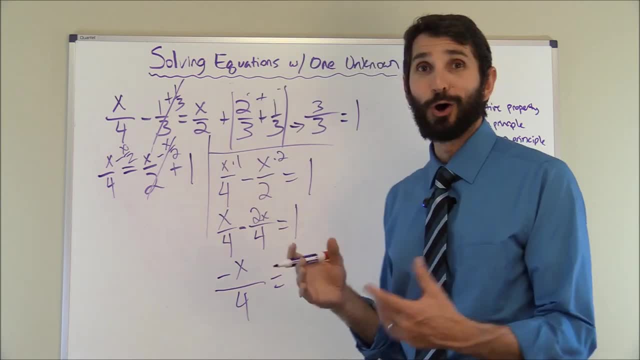 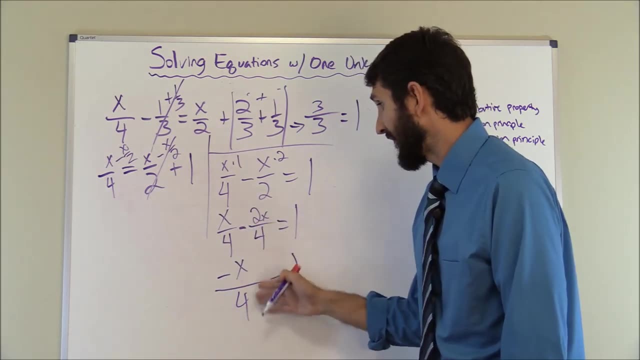 over 4 equals 1.. Okay, we're almost done with this equation. Now, again, we're going to use the multiplication principle because we want to isolate this x on one side and get all the numbers on the other. And the way we do that is since 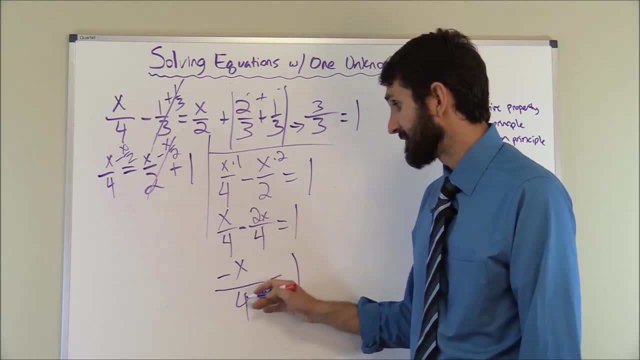 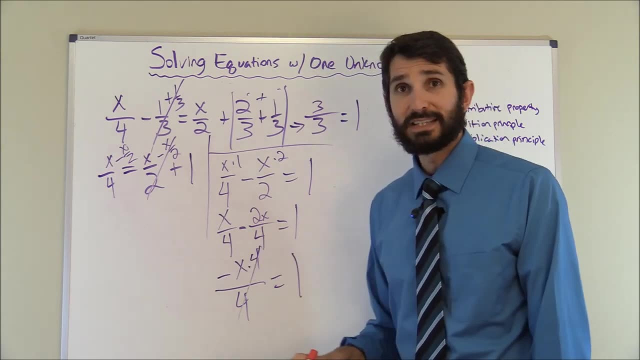 this is a division problem. we're going to multiply, So because it's dividing by 4, we're going to multiply that top number by 4 and that is going to help us cancel that out. But what we do to one side we got to do to the other And we 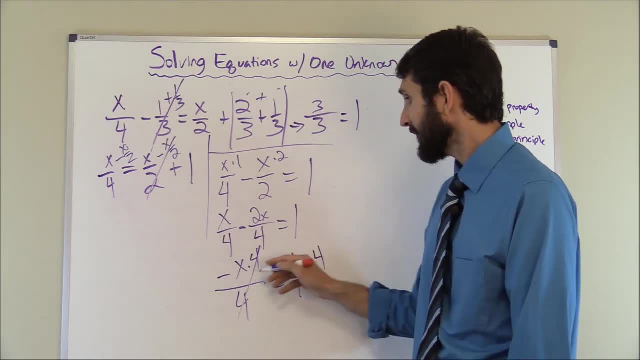 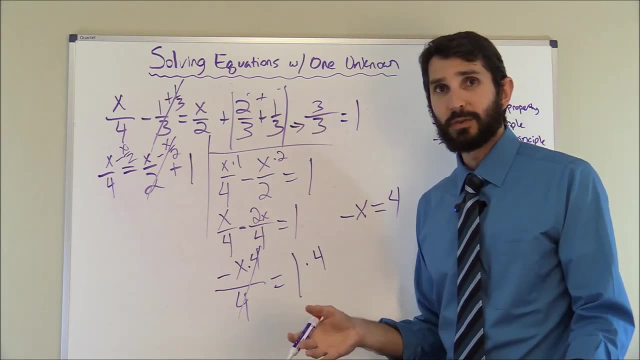 just have a whole number here, so we'll just multiply that whole number by 4.. And what we're going to have now is negative x equals 4.. Now, whenever you are done with the equation, usually you want the variable to be a positive number. 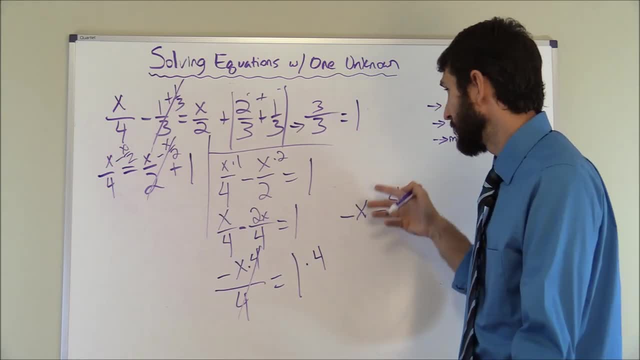 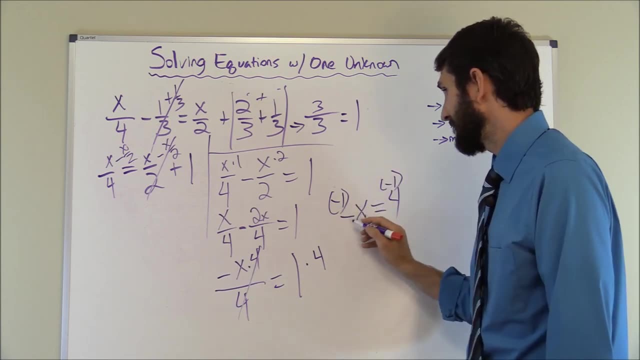 and if there's any negative number, you usually want to move it to this end. so all you do is basically you can multiply that by negative 1 and multiply this one by negative 1 and that will make that a negative times. a negative will give you. 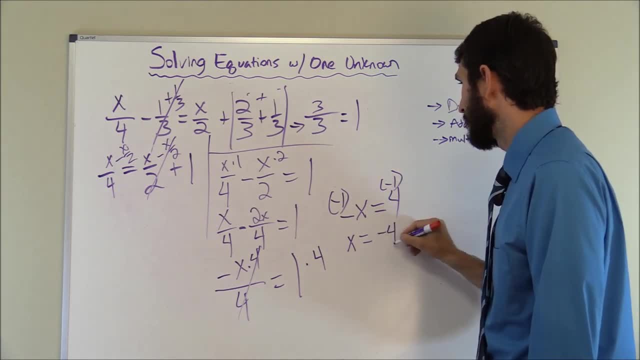 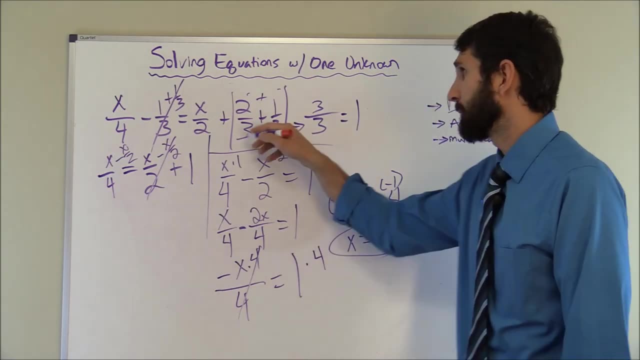 a positive and negative 1 times 4 will give you negative 4. basically you just flip it, so if it's negative X equals 4, it'll be X equals negative 4 and that's our answer. and again we can go back and you can plug that in and you can check. 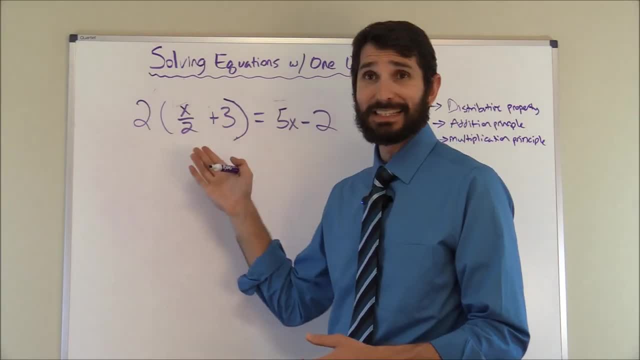 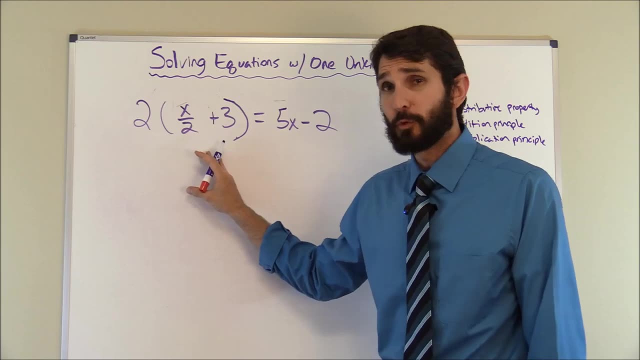 it. okay, I'll show you how to work one more of these. and it has parentheses, it has a fraction, it has everything, but we're going to use those exact same principles and it will be easy. so what we want to do first is get rid of the. 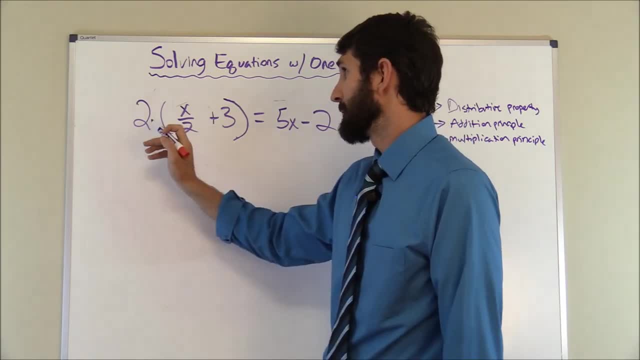 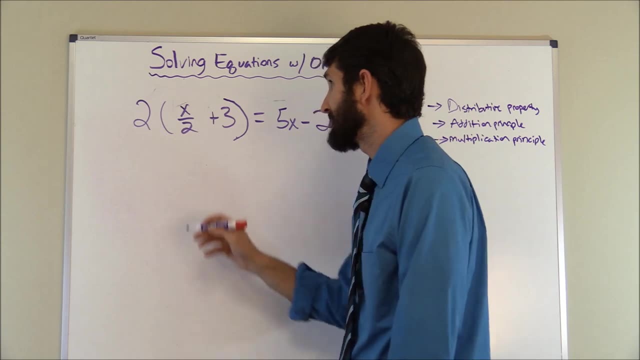 parentheses. and we do that by using the distributive property, which is going to be multiplying 2 times X over 2, and then carry down the plus sign, and then 2 times 3 is going to give us 6. so that's how we're going to do that. so how do we? 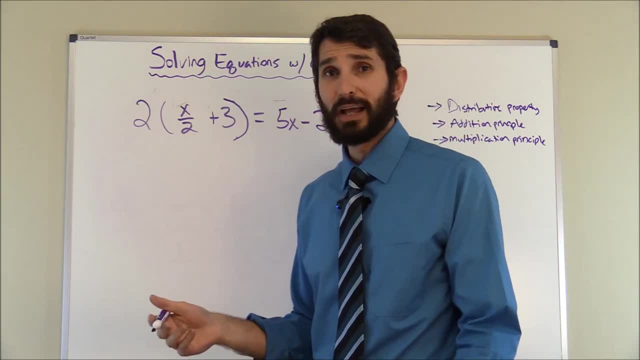 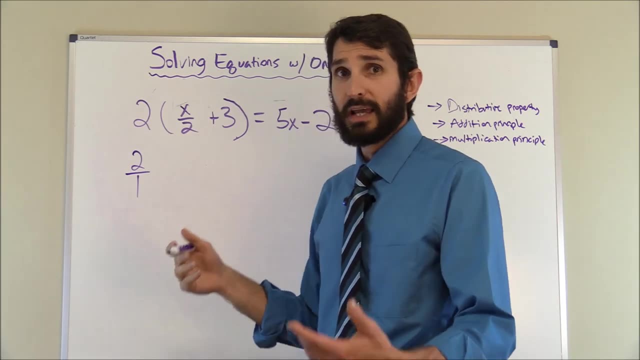 multiply 2 times X over 2. basically it's just multiplying fractions and I have a video on how to do that. but basically I like to set it up like this: 2 over 1, because 2- a whole number is- can also be extremely important. so I'm going to go ahead and show you how to do that and 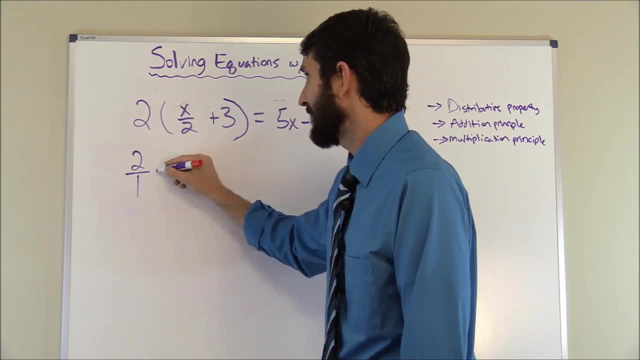 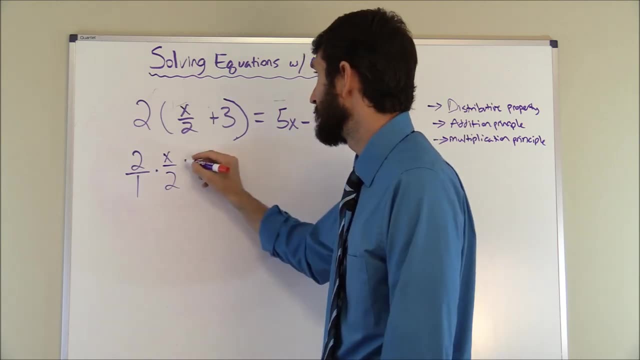 I'm going to go ahead and show you how to do that and express as a fraction by simply putting it over 1. I like to do that because it keeps me straight times X over 2. we just multiply across the top and multiply over the ball across the bottom, and we're done so. 2 times X equals 2 X 1. 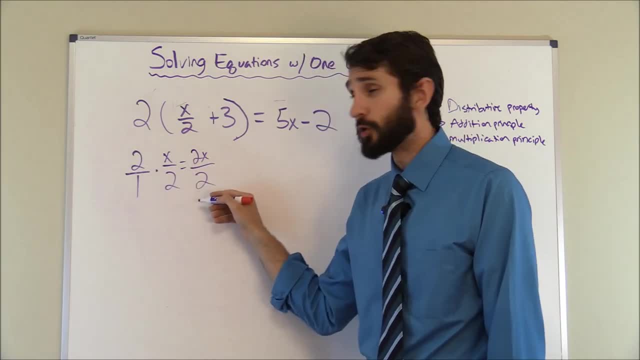 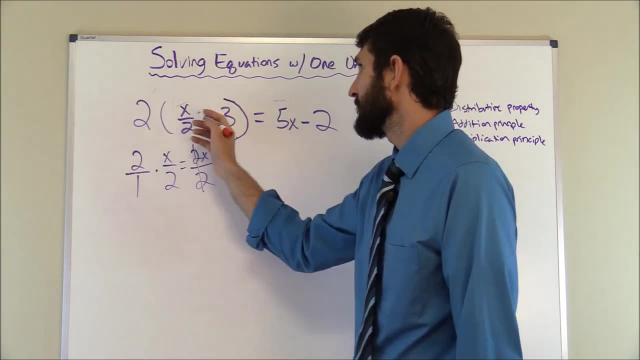 times 2 equals 2, so it's going to be 2 X over 2. but because those numbers are the same, we could actually cross those out and have just X. now we'll make things easier. so 2 times X over 2 equals X, and then plus 2 times 3 equals. 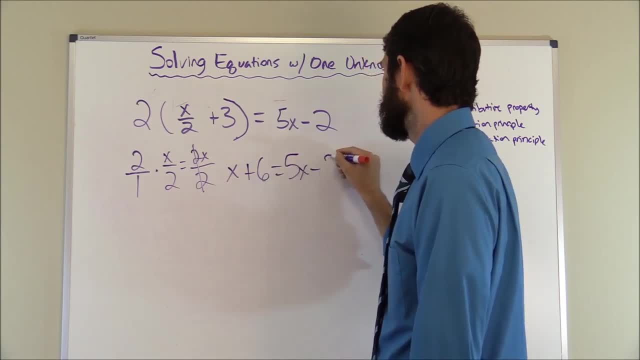 6. so that's how we're going to do that. so that's how we're going to do that. so this is x minus 6, and then equals 5x minus 2. now to get rid of this 6, here we're going to use the addition principle, which states that we do the 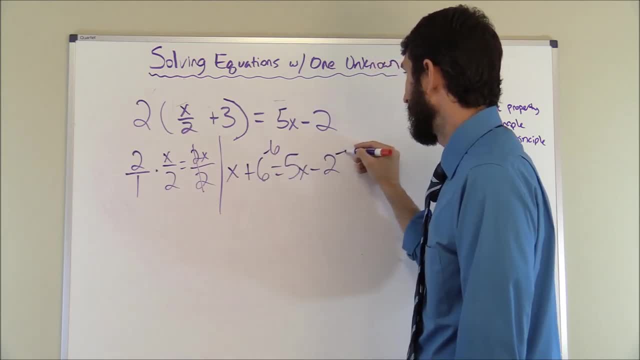 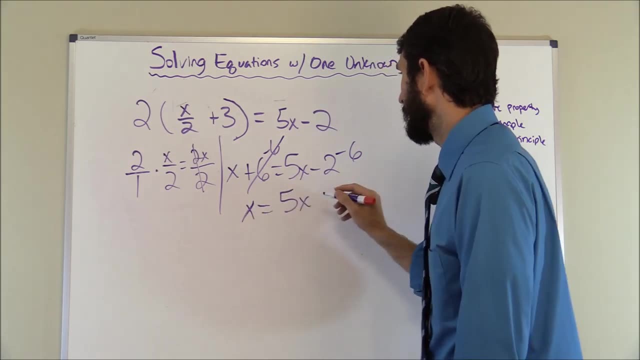 opposite. on this side it's a positive 6, so we're going to subtract 6, but we got to do it to this side as well. that'll cancel that out. we'll be left with an X equals 5x. Okay, negative 2 minus 6 is going to be. 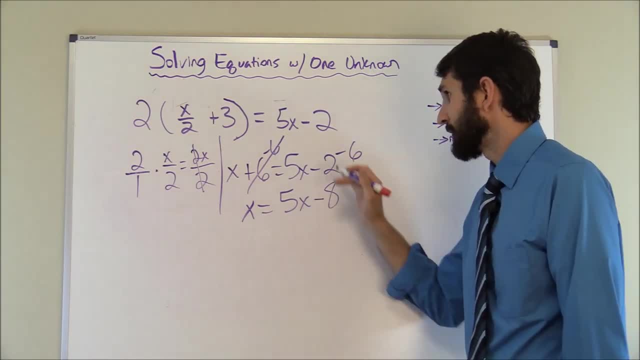 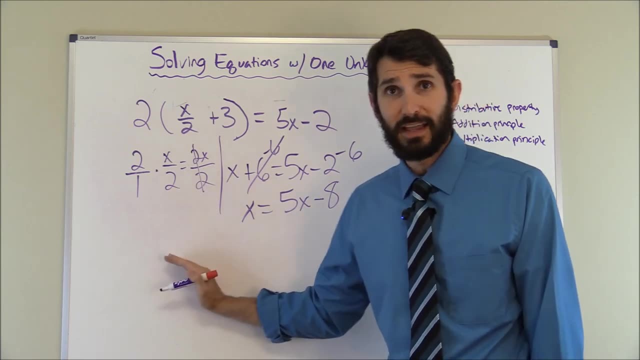 negative 8, so it'll be 5x minus 8.. You always want to keep your negative and positive signs straight, because that's an easy way you can mess up. Now we want to get this 5x over to the left side, and to do that again, we use the addition. 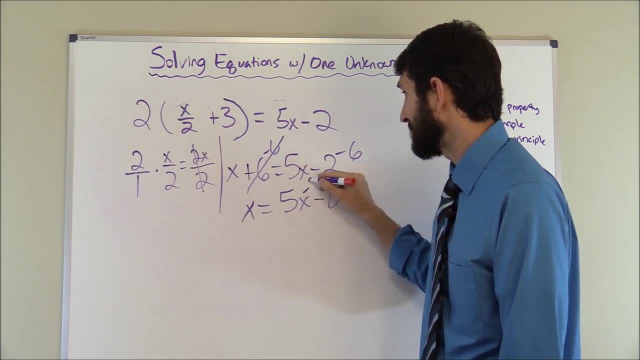 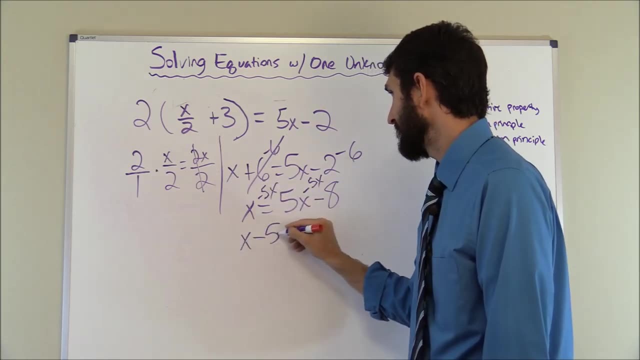 principle. So it's a positive 5x. so we're going to do a negative 5x or subtract 5x. While we do that side, we also go to do that one. so it'll be x minus 5x equals negative 8.. Okay, now again.